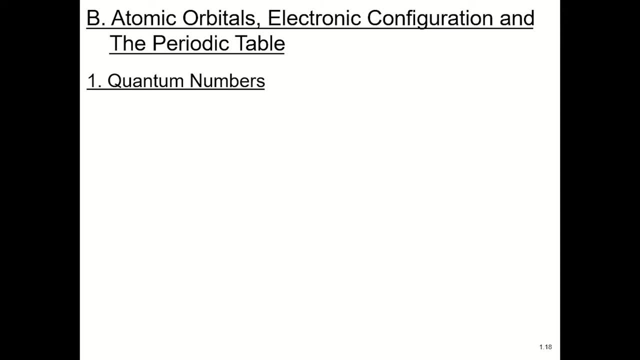 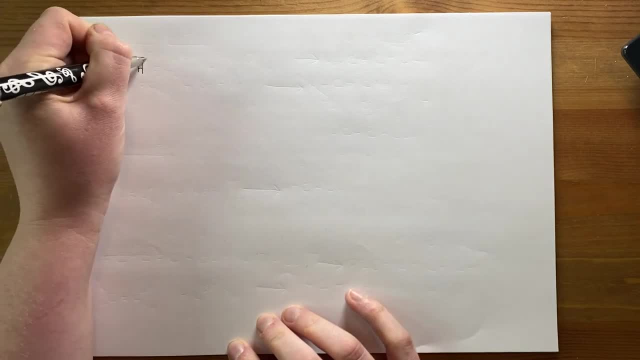 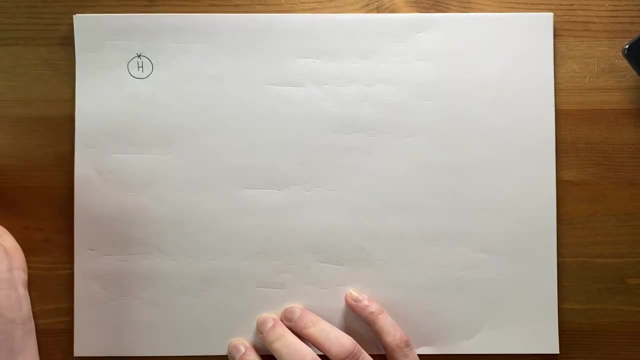 So, if you have a think way back to National 5, which seems like ages ago from now, we always have represented our elements, So say hydrogen, with a nucleus in the middle represented usually by its symbol and the electrons sitting outside the shell like this: 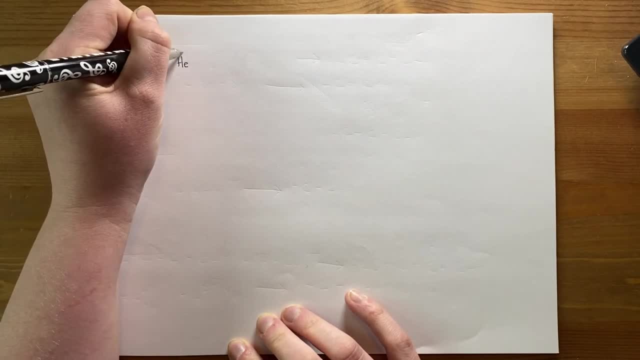 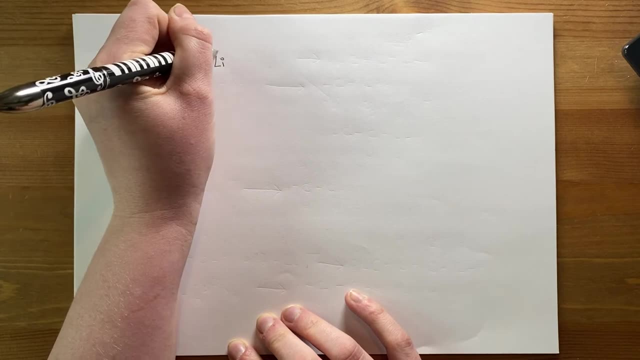 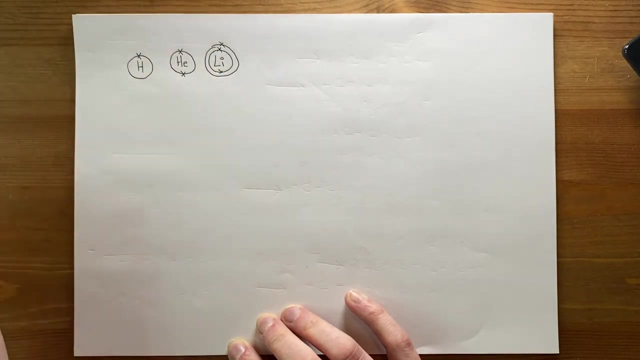 You would get to helium, that would fill its first shell, it would have two electrons And thinking about lithium, it ends up having a second shell of electrons to fit the third electron in. And we keep going through that, through the periodic table. 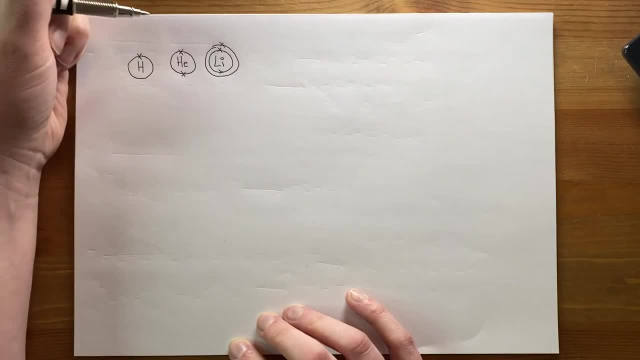 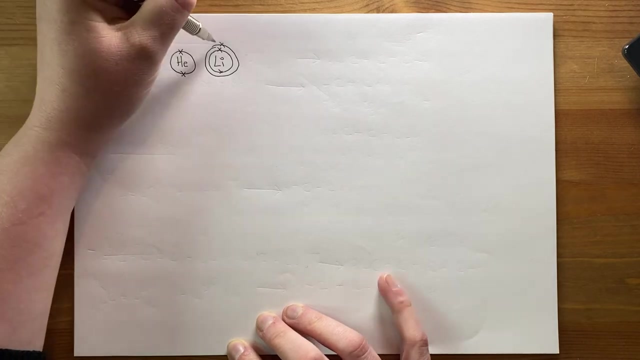 We add shells. the second shell, we said, could hold a maximum of eight electrons, same with the third, and so on. Now, this way of representing our element is fine in terms of our understanding that these different shells exist. It's not quite what's actually there. 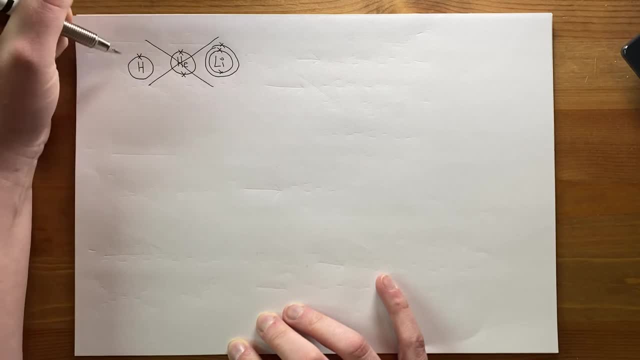 So we're not going to be using this anymore. We're not going to be thinking about our elements in this particular way. We're going to start thinking about quantum numbers. We're going to think about different types of orbitals That these electrons fit into. 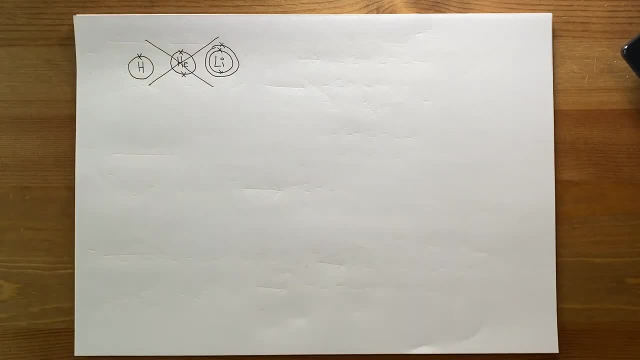 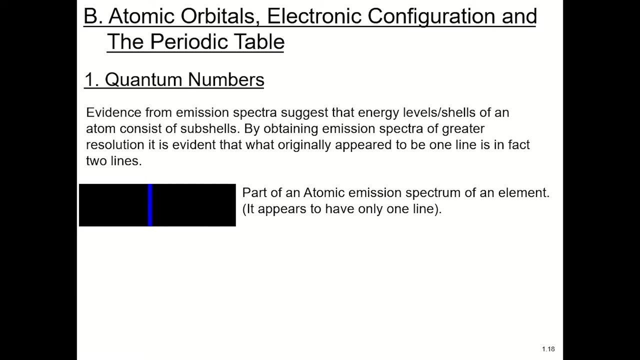 So what we need to do is we need to have a think about our quantum numbers, what these are and how they came about. So we spoke about our atomic emission and absorption spectra. before And from these emission spectra, what they actually found was that the band that you can see on the slide here didn't actually just exist as one solid band. 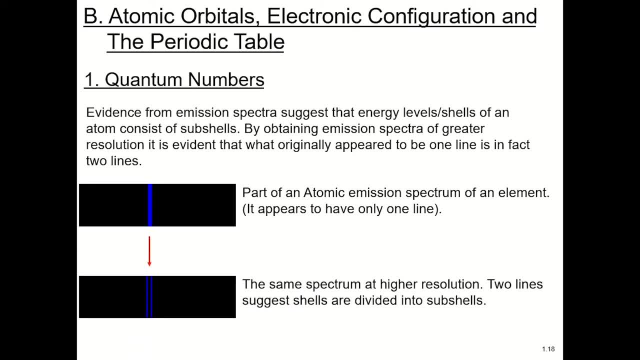 It looks like it's only one line, But if you look at it in a higher resolution, if you look at more powerful equipment to look at the emission of this particular element, you can see that this spectra actually has smaller lines within it, And this was our, if you remember. these were caused by the jumps from our electron from higher to lower energy shells. 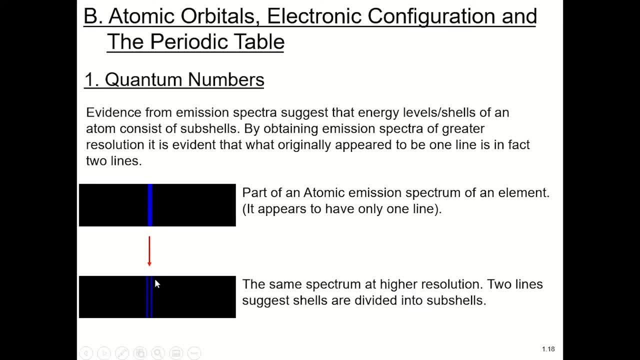 They were emitting photons. What we're seeing in the second one here is that they're very similar, very close together, But this suggests two different jumps, two different jumps back down. If it was in the visible, remember that comes down to the second energy level, second shell. 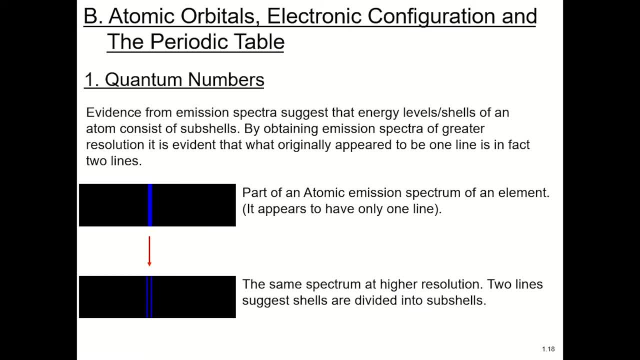 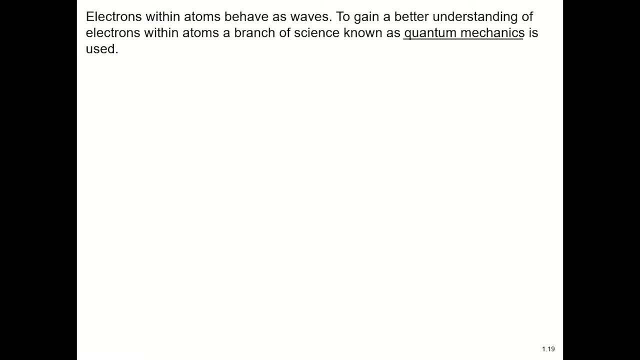 And so they wanted to have a look and see what this actually meant inside. And so, in order to think of this, we think that electrons within these atoms can behave as waves, And really understanding this as a branch of quantum mechanics- Now, don't freak out. 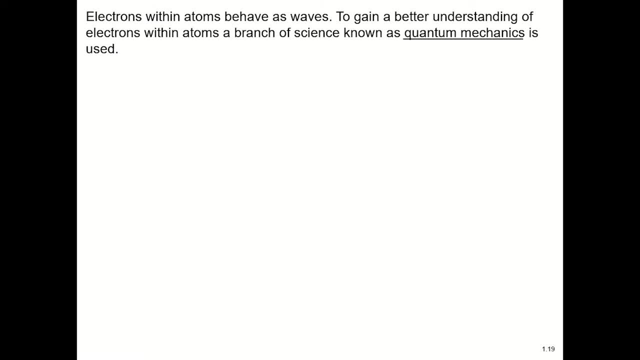 Don't freak out at the fact that we're talking about quantum mechanics. There's only a small part of quantum mechanics we're really looking at in terms of entire chemistry, But there are a few rules that we need to know to be able to identify these electron sub-shells that we want to speak about. 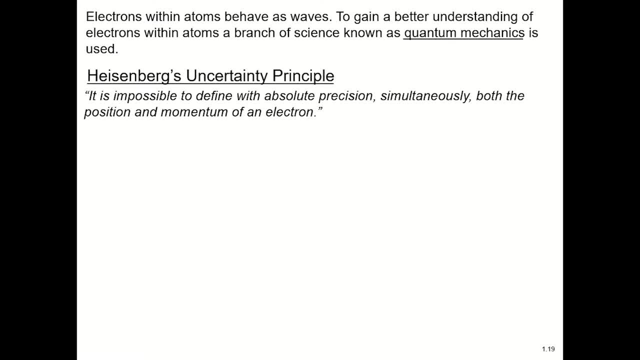 So Heisenberg's uncertainty principle. It's impossible to define with absolute precision simultaneously both the position and momentum of an electron. So we can either know where the electron is or how fast it's going. We cannot know both. One very interesting thing in here: 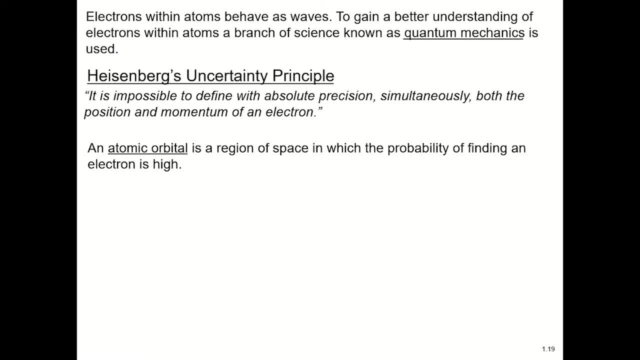 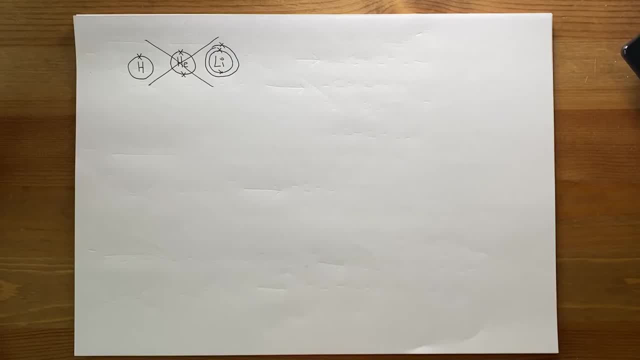 What I want to do is I want to define these orbitals. So the orbital that we talk about is the area in which you are likely to find the electron. So if you have a look in the window, there's a wee sketch of my classroom just now. 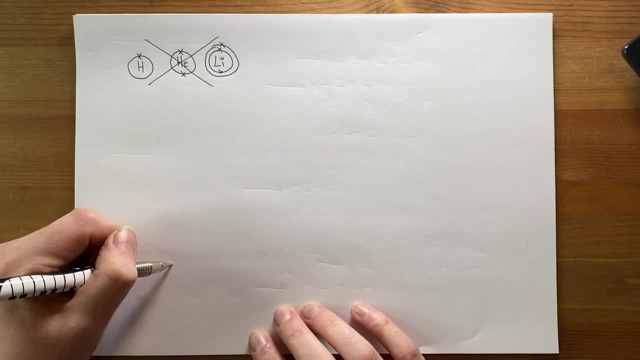 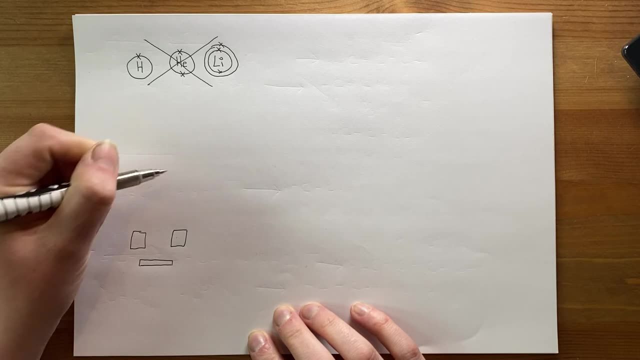 Because normally if I was in the classroom I would be walking about like a lunatic at this point. So my desk in my classroom is at the front and I have groups of desks. I have four groups of desks In my classroom Now I'm quite active. 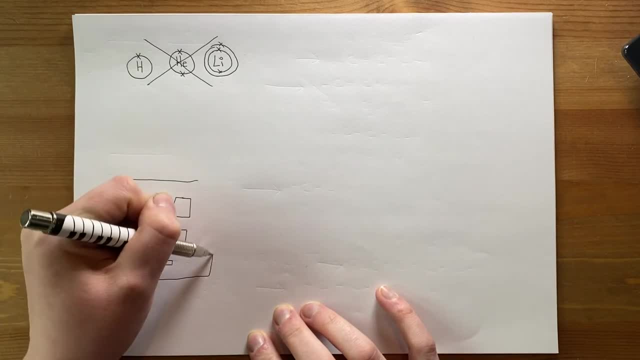 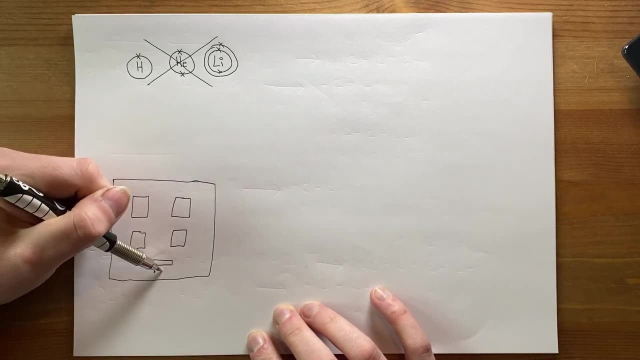 I wander around. So if we say this is a room, there's benches around the side, We won't draw them in. But this is my desk. Normally I would be teaching here, But throughout the lesson I'll be coming out from behind my desk. 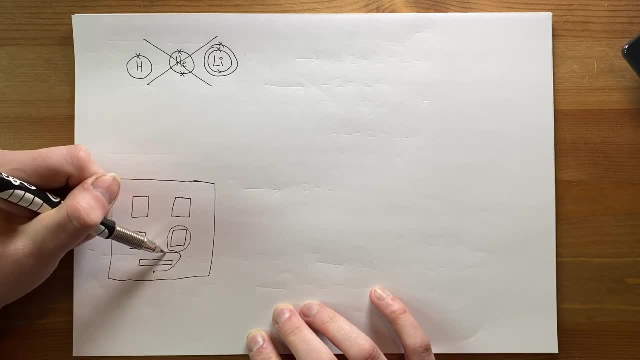 I'll be coming around. I'll be checking on the people on this table. I will be checking on the people on this table. I will be coming up here as well, checking on the people on this table And, if you were to time, lapse me throughout my lessons. 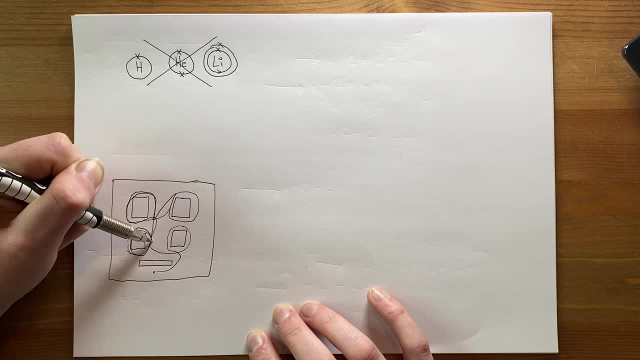 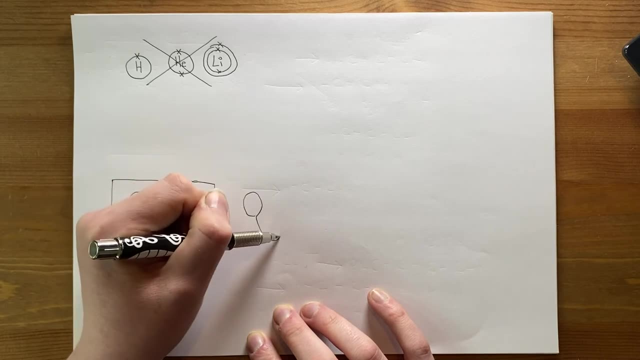 you would find that I seem to go on quite a specific path, And that path has a bit of a shape to it, doesn't it? It's got a bit of a shape, that kind of looks, I don't know like that. 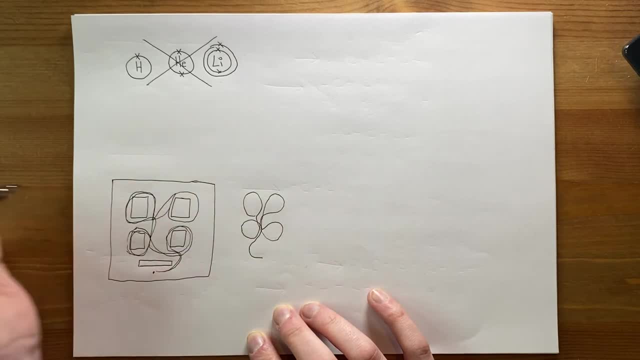 We'll just go with this. Yeah, Let's just say my four leaf clover that I've just drawn there. That's the likely path where you're likely to find me Now. I still might be darting out of the classroom to go see another teacher. 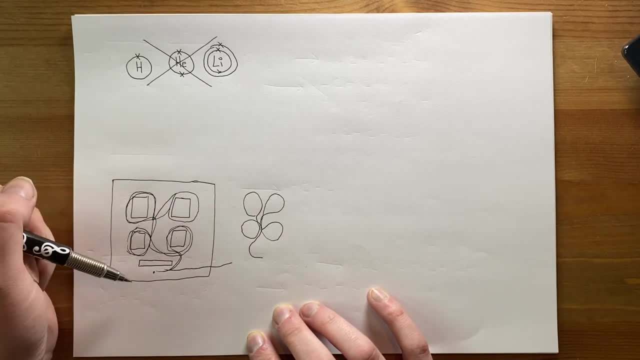 Be back in, But I'm likely to be going in and out and round these desks, These desks throughout. And now this shape is not a physical thing. This shape is a map of where you will likely find me during a lesson when I am teaching. 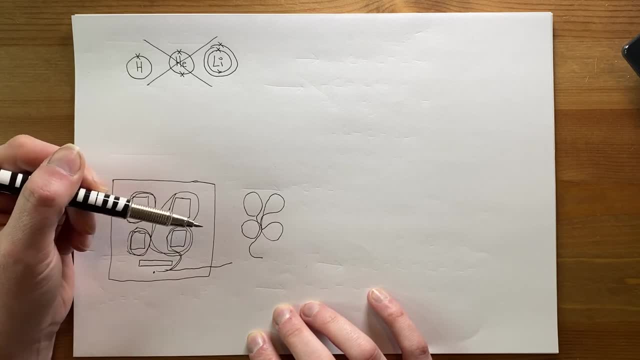 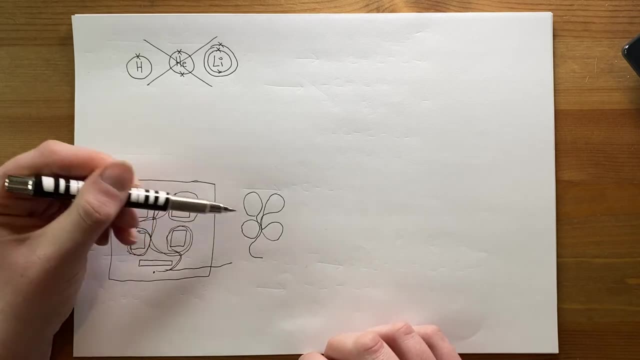 And that's kind of what we're looking at when we're talking about these orbitals, because I'm going to show you some shapes, But it's quite important that you don't think of them as physical things. They are areas where there is a high probability that you will find the electron. 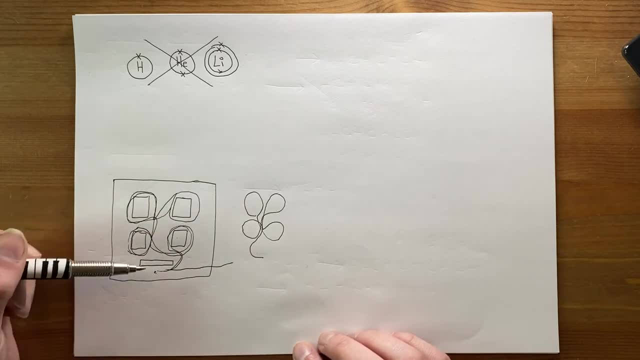 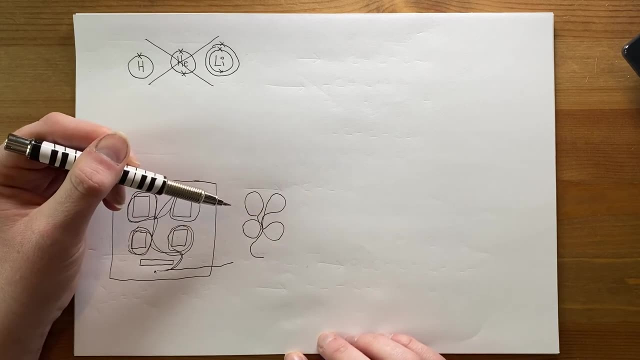 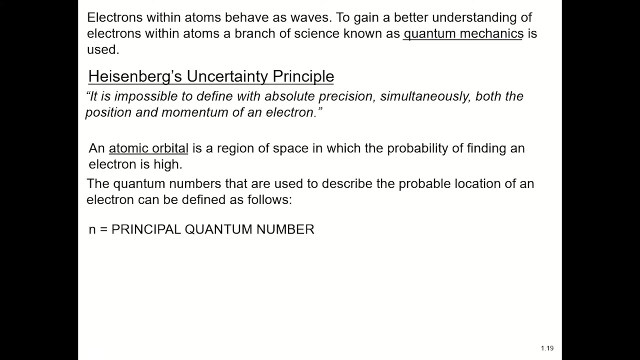 So if this was my atom and I was the electron, then the probability is within this shape, somewhere you would find that electron. That's what we're looking at when we talk about these different orbitals. So, moving on from that and my interesting drawing, 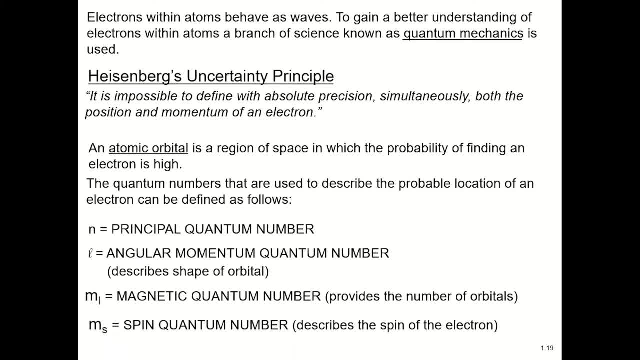 There are four different quantum numbers that we're going to speak about that allow us to determine these shapes and determine which electron we're speaking about, And you can see them on this slide just now. So M is the principal quantum number. L is the angular momentum quantum number. 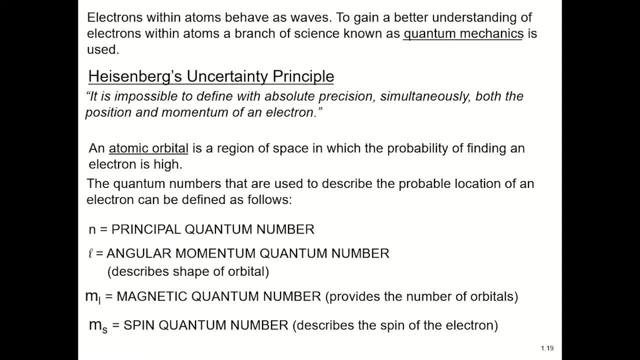 which describes the shape as we're kind of seeing here. M with a subscript L is the magnetic quantum number, which tells us the number of orbitals, And M subscript S is the spin quantum number. Now we'll go through these all individually. 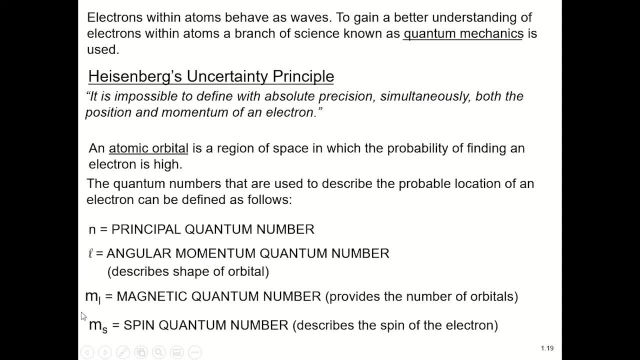 Don't panic with them. What I want to draw your attention to are the last two: The magnetic quantum number and the spin quantum number. Now, the magnetic quantum number- You can just find my mouse. There we go. M subscript L: The SQA last year updated the advanced higher course. 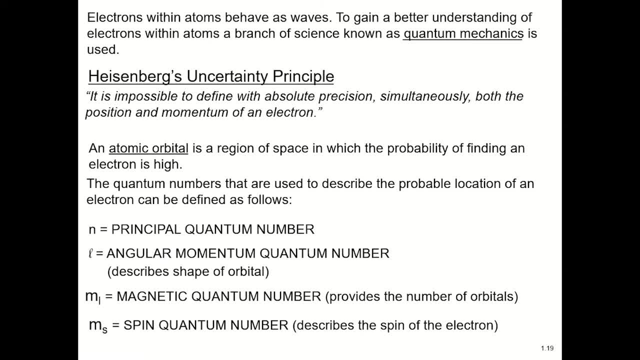 to accurately represent how we represent these things in chemistry. Now this M subscript L. I've lost my mouse again. There we go. M subscript L used to just be represented by the letter M, So if you're looking through any old notes, 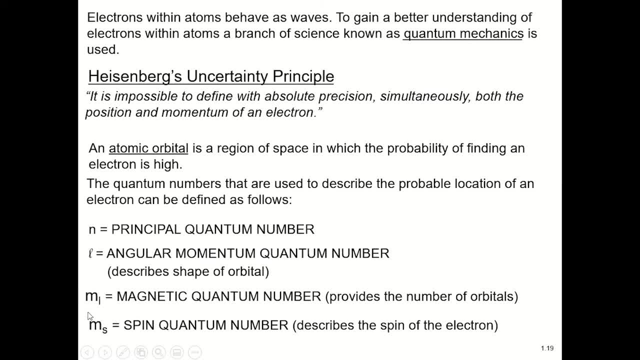 if you're looking through any old textbooks that are for advanced higher chemistry and it says the quantum number M with no subscript, then that is referring to this, the magnetic quantum number that has changed to M subscript L, M subscript S as well. 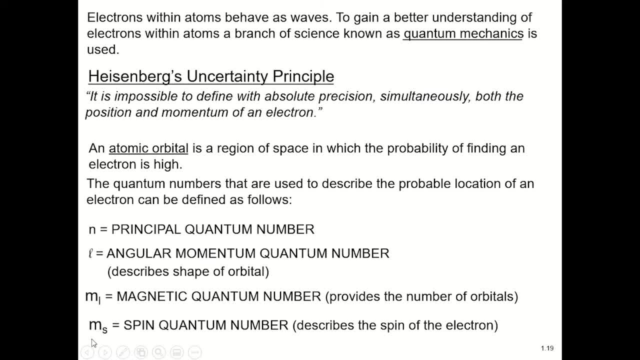 This used to just be represented by an S. Now don't ask me why this all got updated. It caused lots of confusion. But when you are looking at old questions from past papers, when you are looking at old textbooks, old notes, this would have been M and this would have been S. 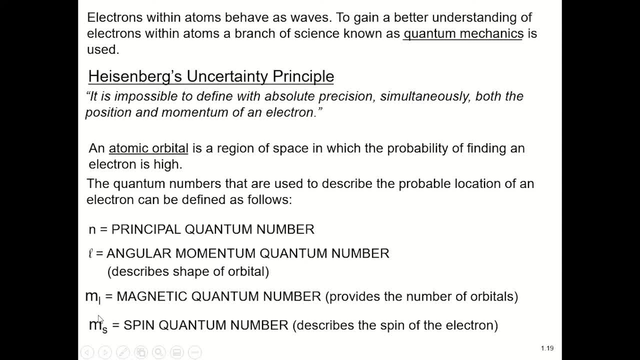 This is the correct one. This is the correct way to represent it Now: M subscript L and M subscript S for the magnetic and the spin quantum numbers. Now we're going to go into what these actually are, but that's really important information. 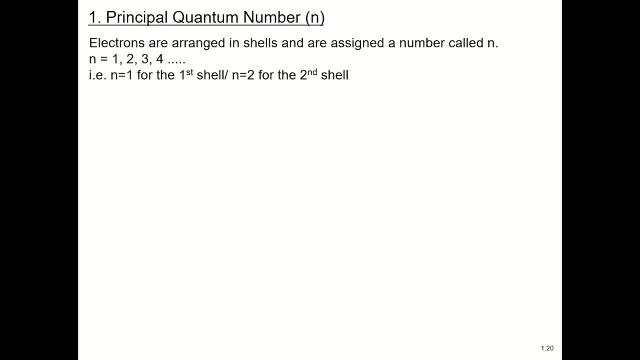 So let's have a look at the principal quantum number. What I said earlier about our different shells- and that's strictly not true, We still have these energy levels. We still have shells: the first shell, the second shell, the third shell. 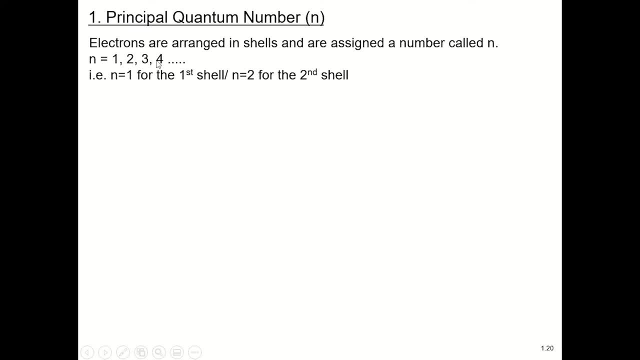 and the nucleus. It's just that within these shells there are these other shapes where you will find the electrons, if that makes sense. So in terms of the principal quantum number, it's quite easy to remember. The principal quantum number N equals 1 for the first shell. 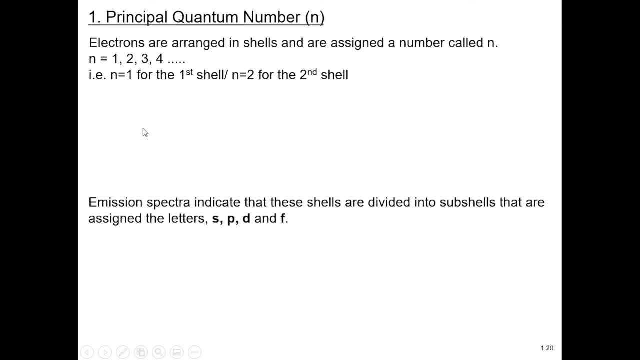 N equals 2 for the second shell, and so on. These emission spectra, however, because it's been further subdivided, allow us to think that actually these shells can divide into sub-shells, and that's where our other quantum numbers come into play. 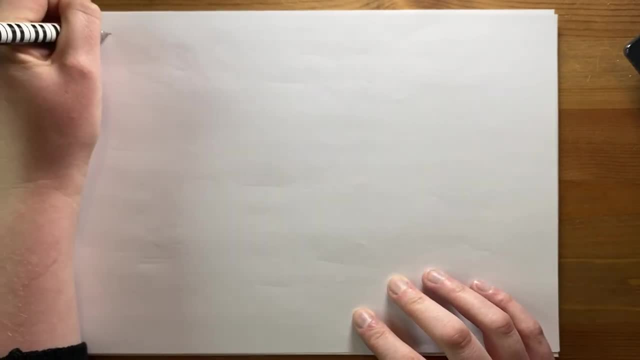 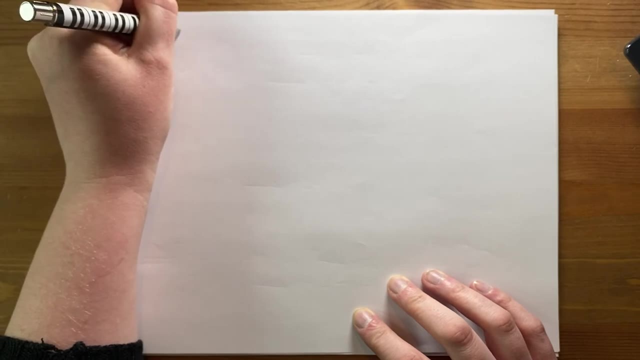 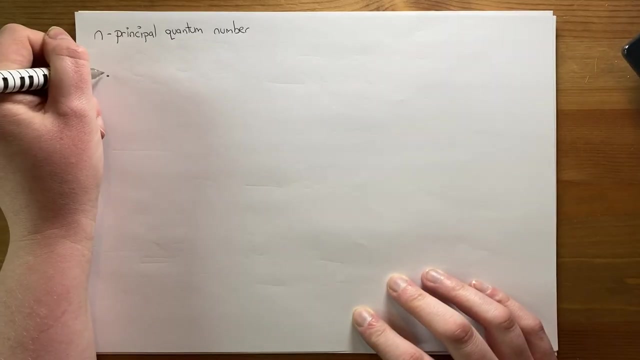 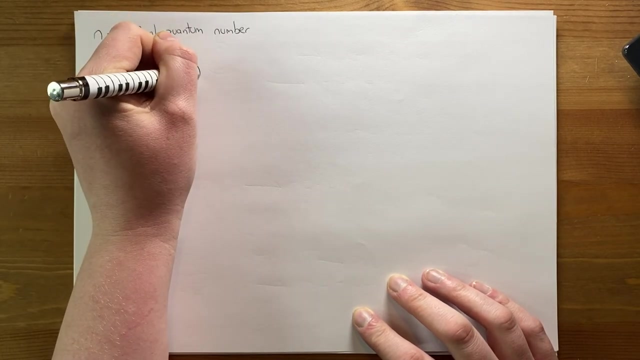 So just looking at the paper just now, if I'm talking about N, which is the principal quantum number, that is, if you have your nucleus, you have your first shell, so N equals 1, and then you would have say a second shell here. 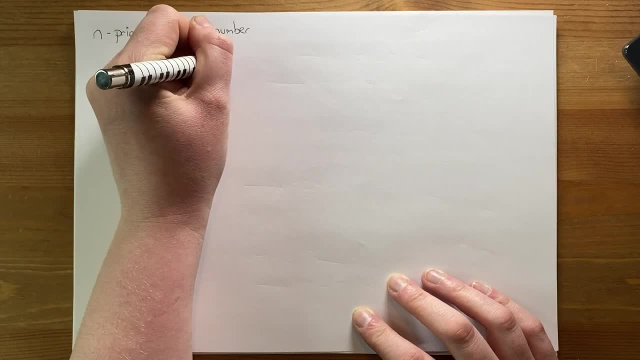 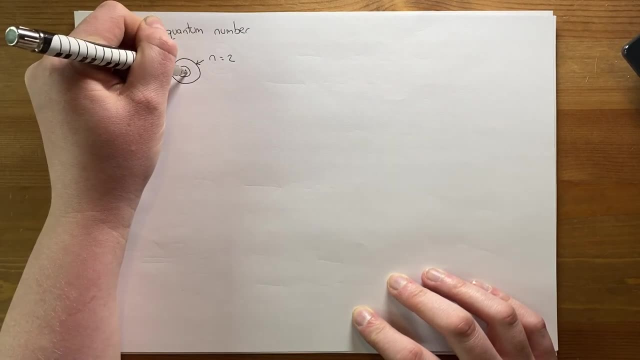 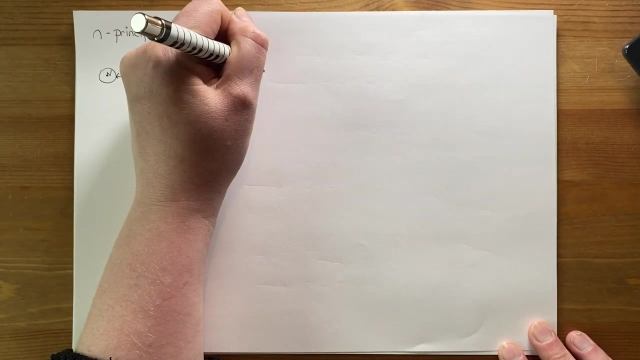 So this shell here would be: N equals 2, and so on. So essentially, this would be your nucleus: N equals 1, and N equals 2, and so on. You would then also have your N with your third shell. 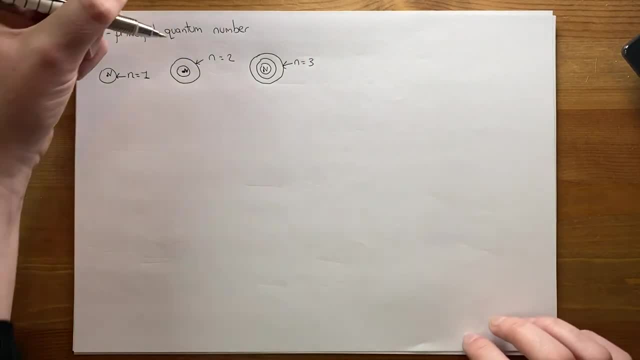 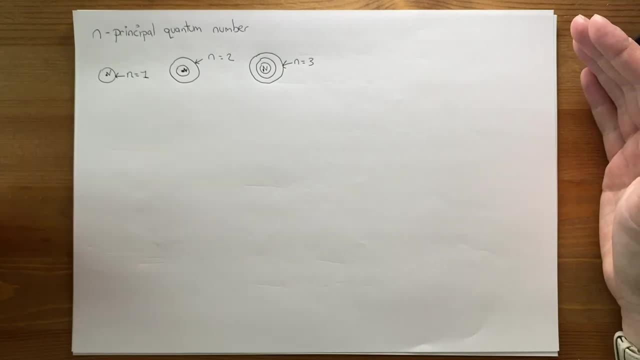 This would be N equals 3.. Now I just represented these as circles just now. I know I said that's strictly untrue, but we're just looking at these as different levels away from that nucleus. Now we're going to look into those levels. 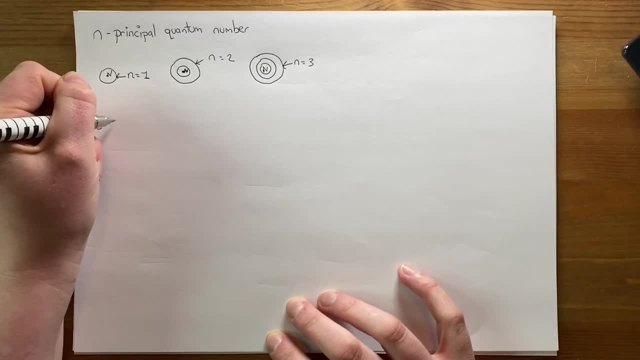 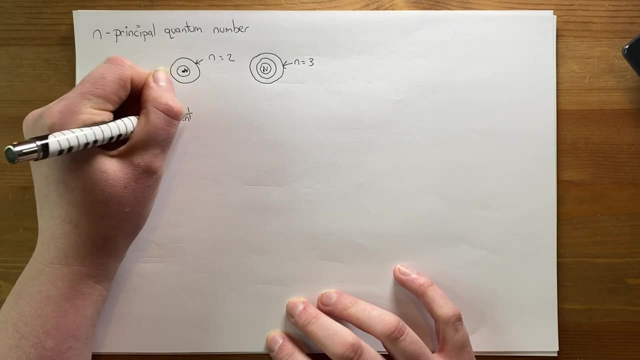 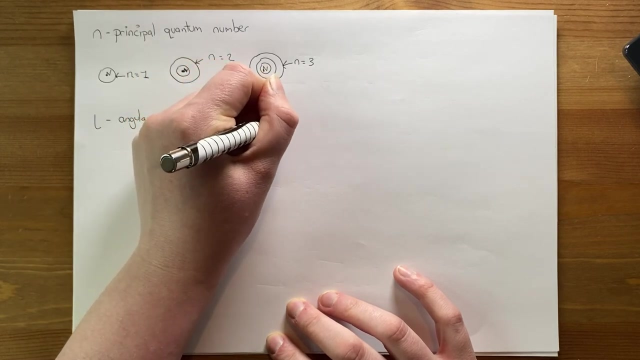 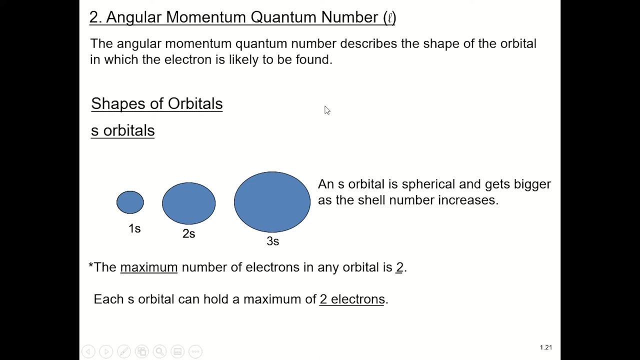 We're going to have a look at L. Okay, so we're going to have a look at the angular momentum quantum number. So the angular momentum quantum number, if we have a look at the slide, tells me about the shape. So this equals the energy level. 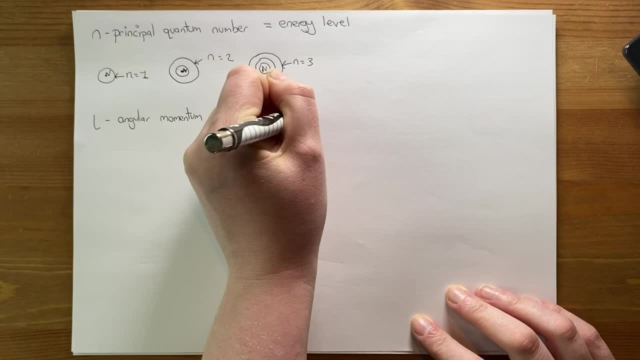 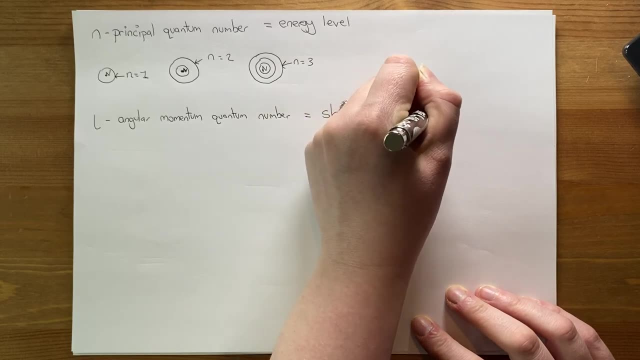 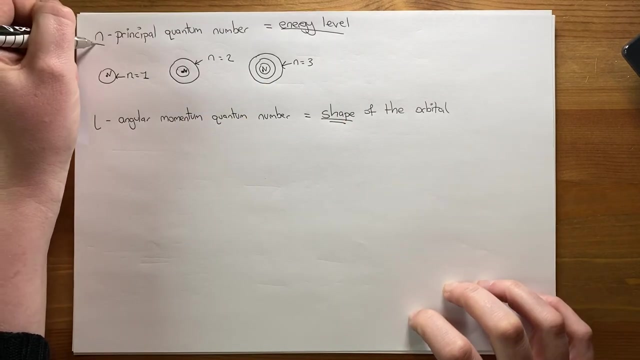 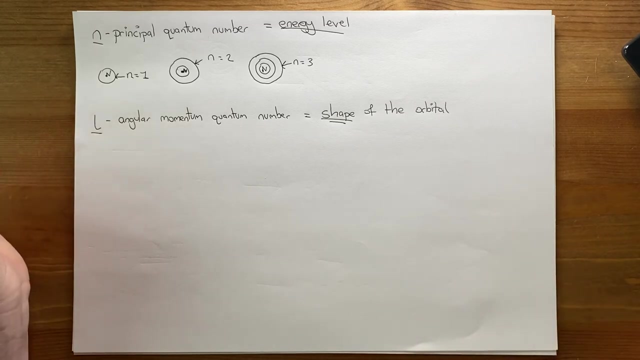 if you like the first one, This equals the shape of the orbital. Okay, so N is the energy level, L is the shape of the orbital within that energy level. There are multiple that you can use. You could get. there are a few. 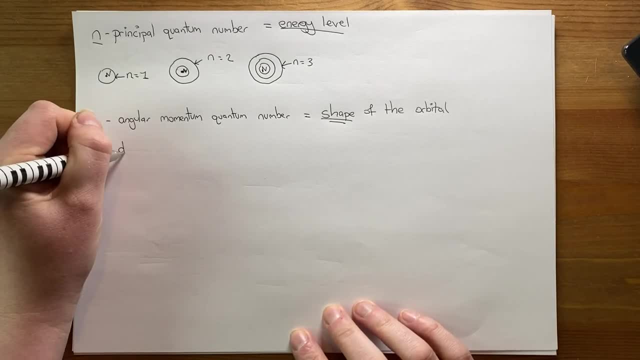 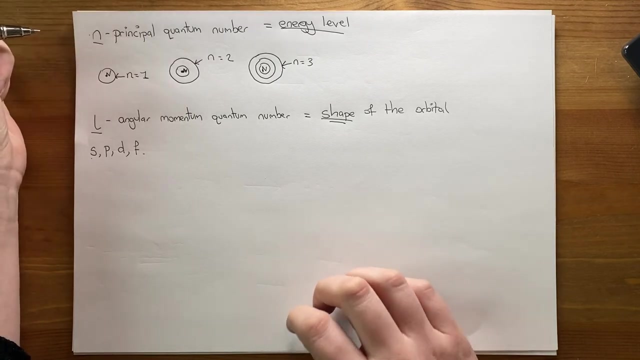 So there's S, P, D and F- These are essentially the names that we give the different shapes that you can find of these orbitals- And these are determined by the principal quantum number. All gets very, very confusing, So. 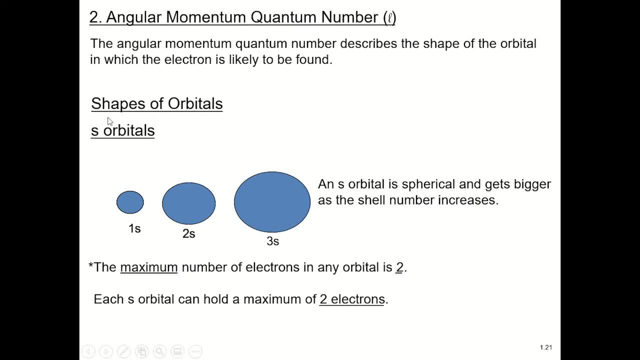 let's start with an S orbital And you can see this on the slide. I'll draw some other ones up in a second. But back to the slide. if we have a look, the S orbitals 1S, 2S. 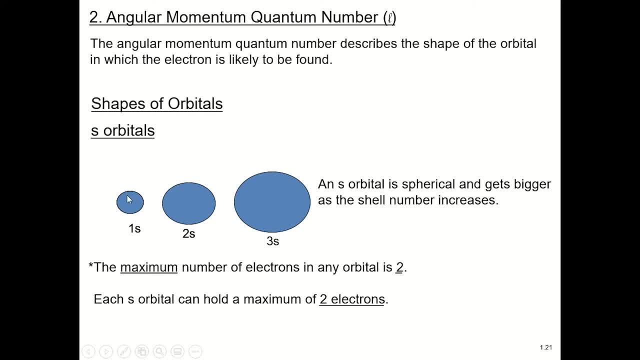 and 3S. here they are spherical in shape. Remember, these are not physical things. These are areas where you're going to find these electrons And as you go to different energy levels. so this would be N equals 1 with an S orbital. 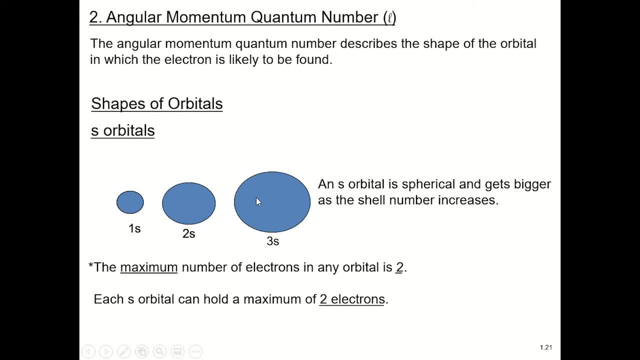 N equals 2 with an S orbital. N equals 3 with an S orbital. they get larger. You can get a maximum of two electrons in these orbitals. So there would be two in the 1S. you can get two in the 2S. 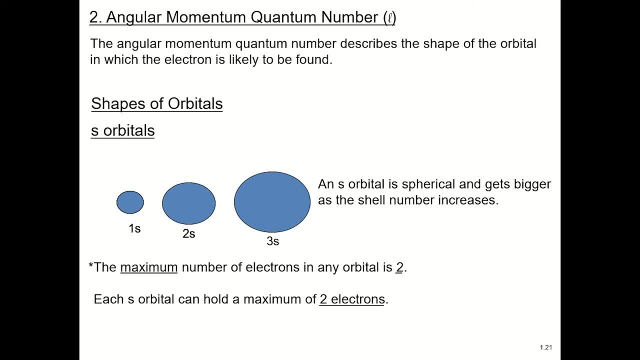 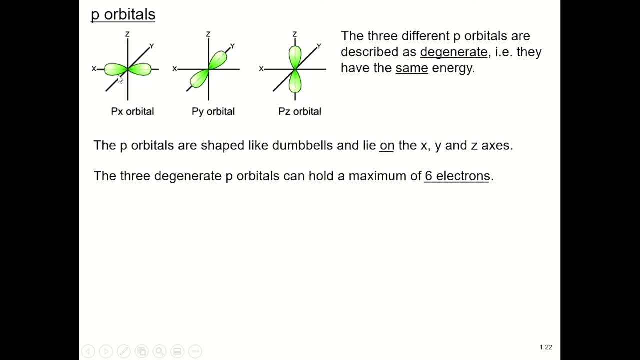 you can have two in the 3S, No more. P orbitals are different, So P orbitals are a dumbbell shape. So you can see here again this kind of dumbbell shape here And they lie on the axes. 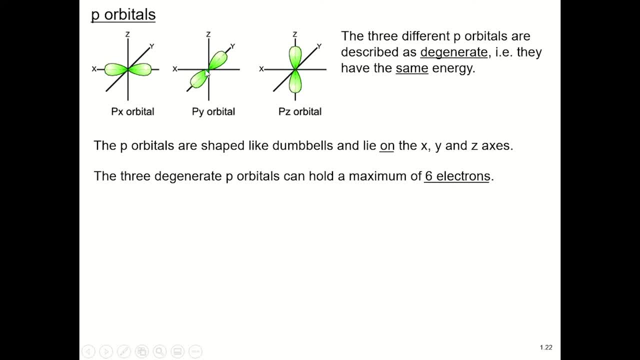 And there are three of these in a shell. Okay, There are three of these in a shell. So there are these dumbbell shape. You can get them on here: the X axis, the Y axis and the Z axis. Okay, 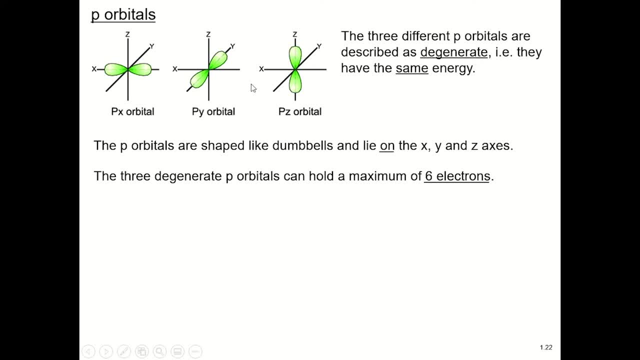 And the word here, degenerate, is quite important. This means that any electron in either of these would be of equal energy. They have the same quantum quanta of energy, So they are degenerate orbitals. Sorry, I keep bringing that menu down. 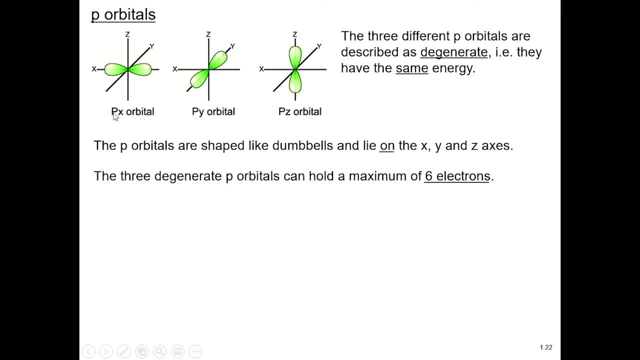 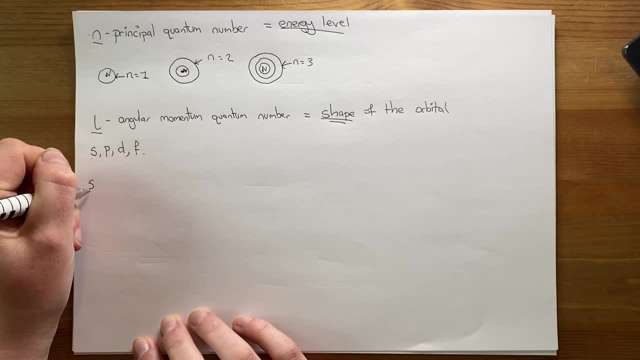 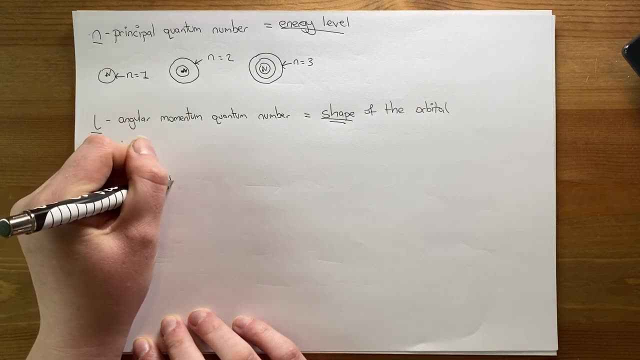 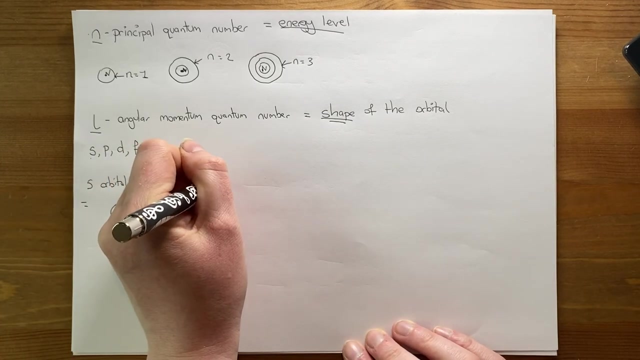 So they lie on the X, Y and Z axis and their names are P subscript X, P subscript Y, P subscript Z. So let me just write this on the paper just now. So S orbitals are spherical, P orbitals are dumbbell shaped. 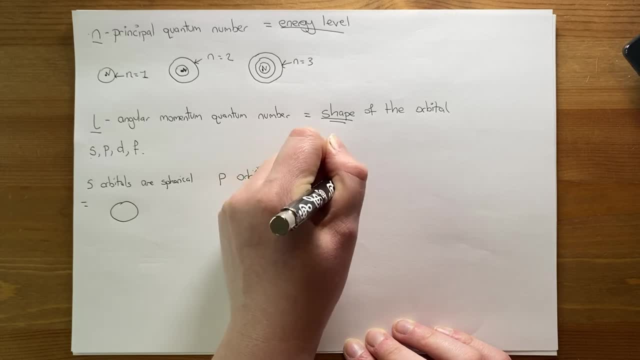 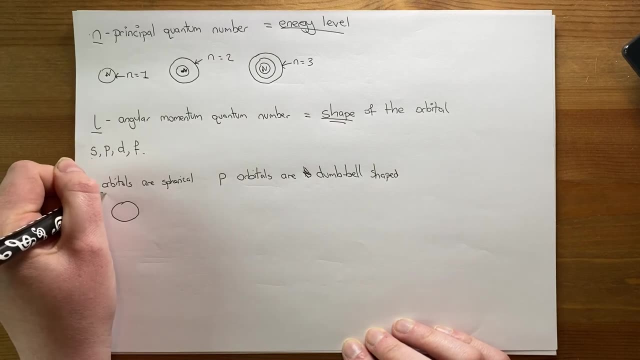 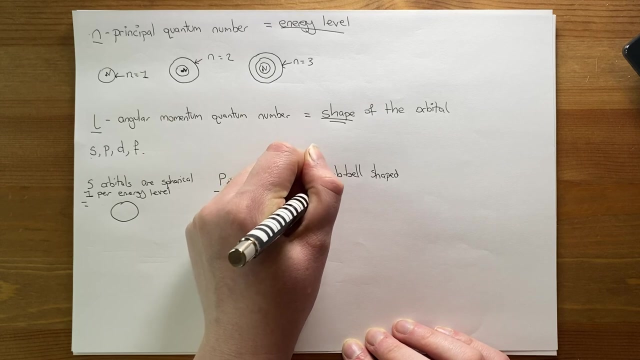 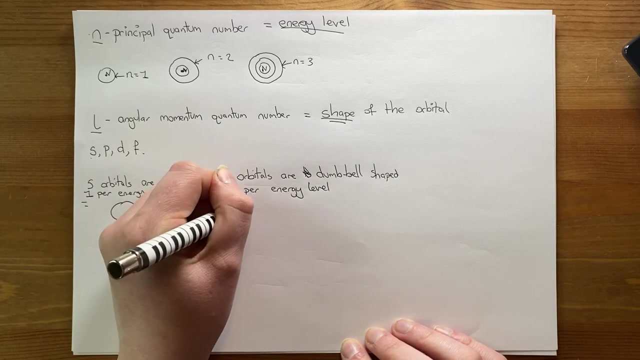 That's not how you spell it: Dumbbell shaped. Here we have one pair energy level, Here you have three pair energy level. So this is X, this is Y and this is Z, If I have this one here on the X axis. 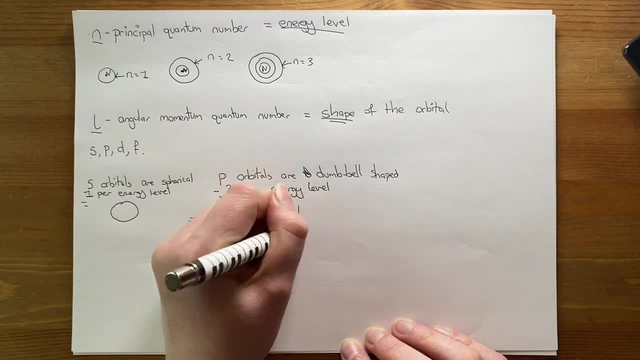 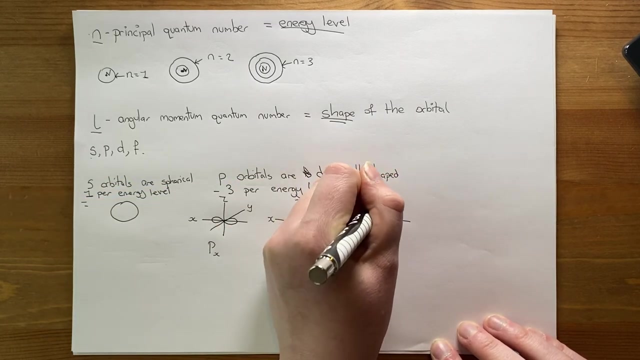 this is P subscript X. I have another one here. I'm just mimicking what we have on the side here. This is going on my Y axis, So this was X, Y and Z. So this is P subscript Y And here. 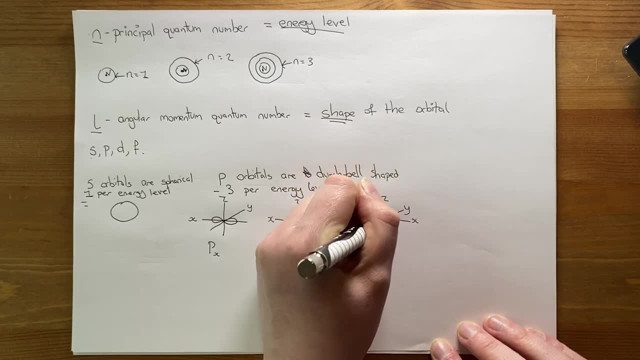 we have Z, where the dumbbell shape is on the Z axis, and that's P, subscript Z. Really important when you're identifying these. you should be able to identify by looking at it that this is PX, this is PY and this is PZ. 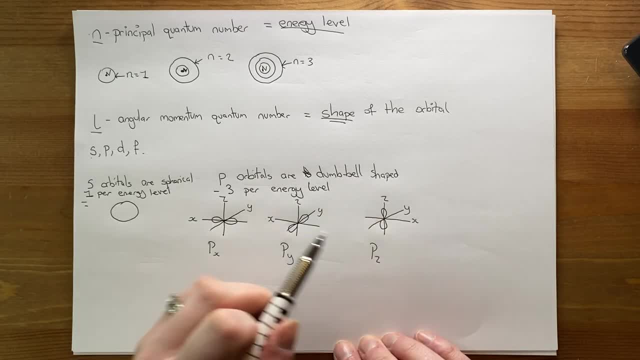 because they're on these axes. You would not be required to know which of these. your electron is definitely in. You just need to know that they exist. But you would be able to draw them and identify them from these diagrams or draw the diagrams. 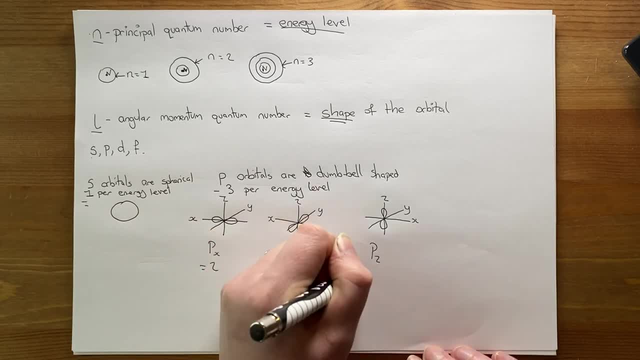 Each one of these can hold two electrons, Six electrons in the P orbitals And per shell or per energy level. So in an energy level, if I've got P orbitals, I would have three of them. They would be degenerate. 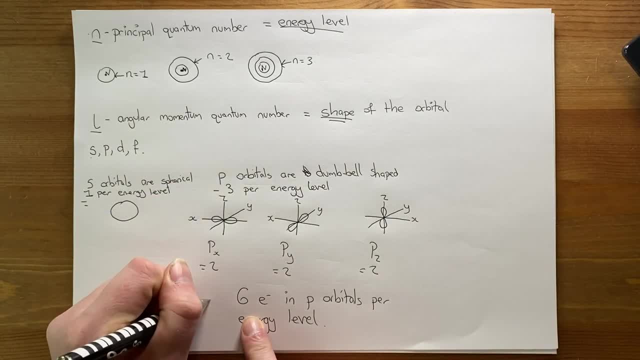 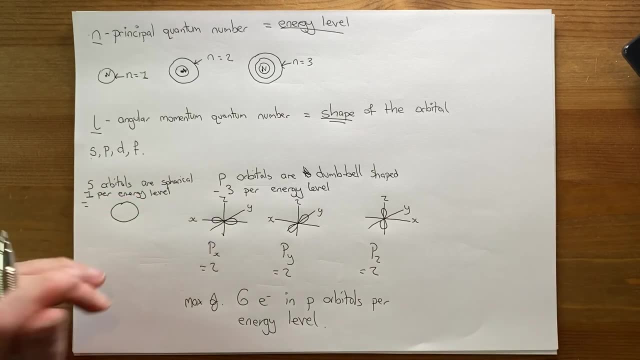 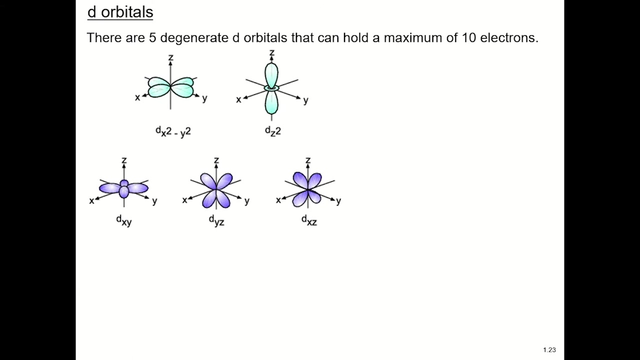 and I can have a maximum of six electrons in those P orbitals, So two each, And we'll talk about that again in a second. Now looking back to the slide, because I am not going to draw these, because they are a pain to draw some of them. 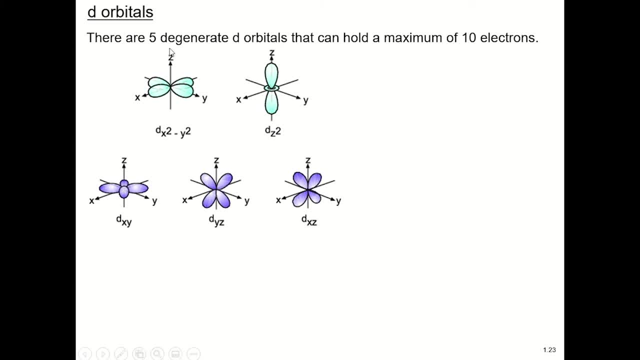 You get d orbitals. Now these d orbitals- again you'll see this word- degenerate. They have the same energy. Each one can hold a maximum of two electrons. So you can now have ten electrons in the d orbitals in a shell. 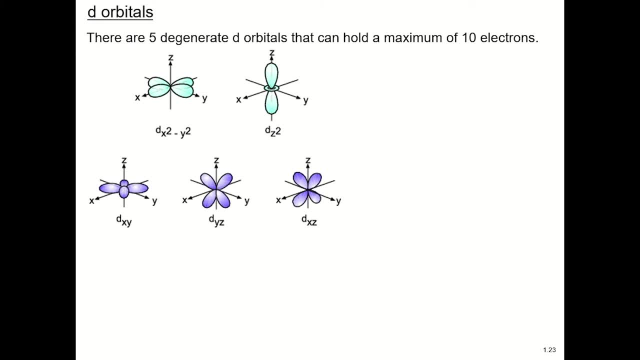 I'll come back to that in a second. You need to be able to identify these. You need to be able to do this one in particular. This is called dz squared. dz squared is the different shape to the rest. It's like a dumbbell shape. 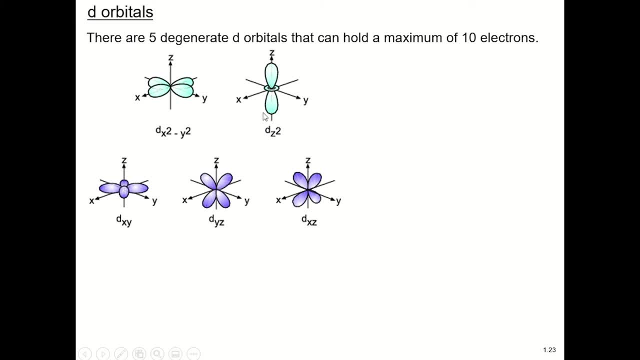 with a donut in the middle So that dumbbell shape goes up and down that z axis with this dumbbell shape in the middle. That is dz squared. The other ones are dx squared minus y squared, dxy, dyz and dxz. 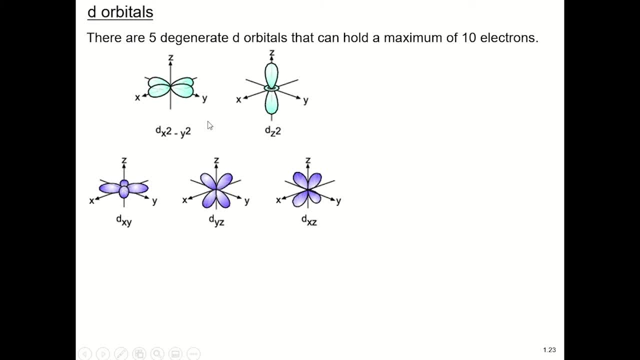 The easiest way to be able to recognise these and know them if there's a squared in its name. so dz squared and dx squared minus y squared, they lie on the axes. So here, this is on the x and y axis, which is why it's dx squared minus y squared. 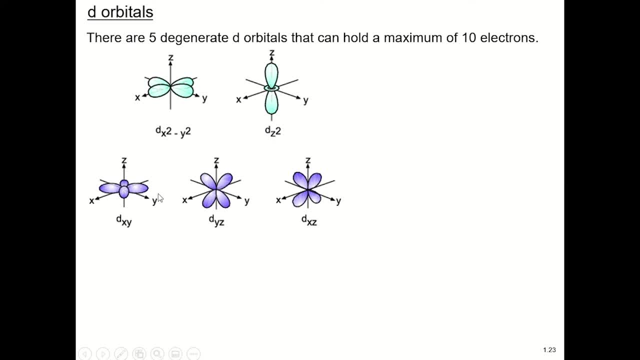 This is on the z axis, so it's dz squared. These ones- dxy, dyz and dxz- lie on the plane of these axes, So this does not go up and down the z axis at all, but it lies in between the x and y. 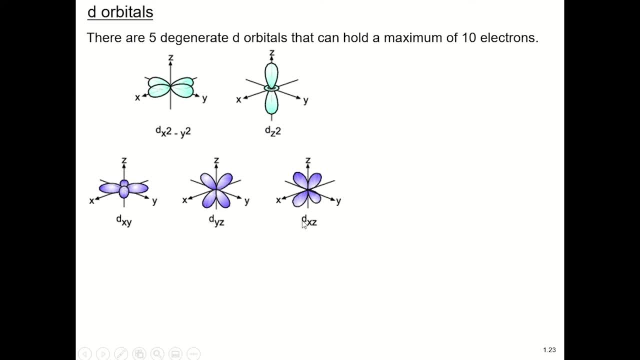 Here this lies in between the y and z, And here this lies in between the x and z, which is why it's dxz, dyz and dxy. They are this kind of double dumbbell shape and they have two each. 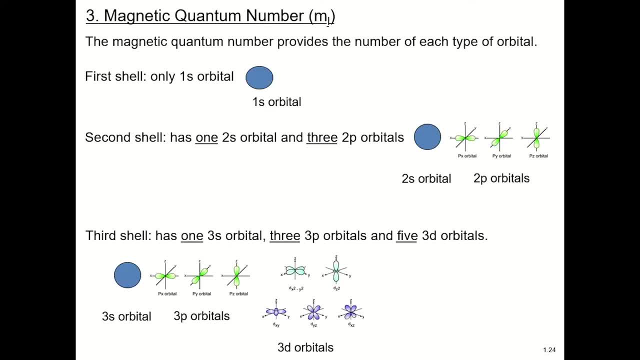 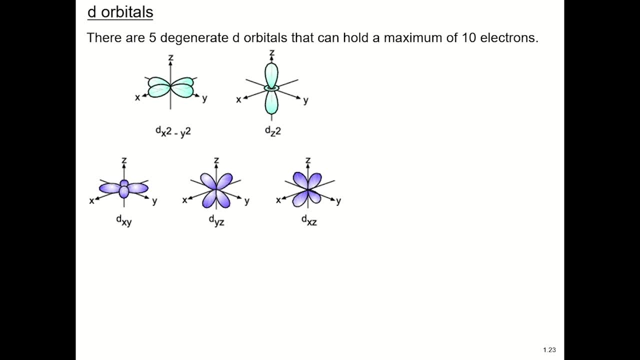 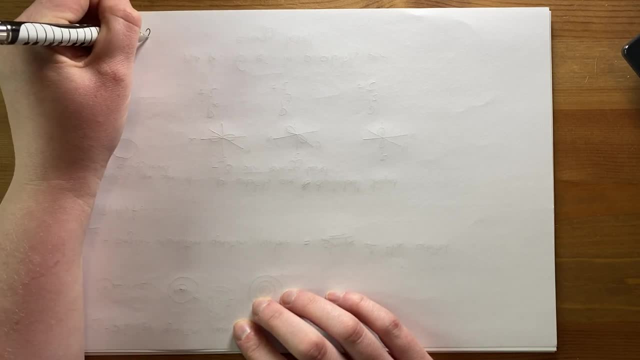 which is 10 electrons maximum in the d orbitals. Okay, Now, if you have a think about how we know how many there are here, in terms of my n, principal quantum number, that equals 1,, 2,, 3,. 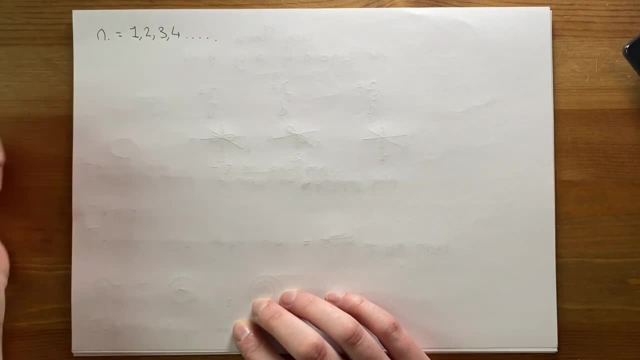 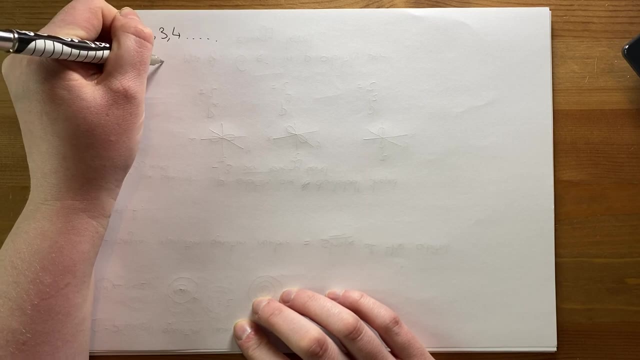 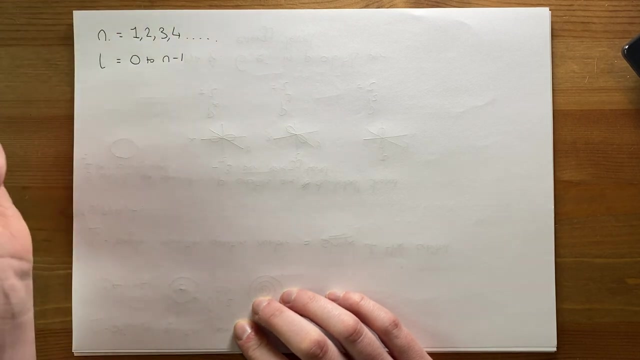 4, and so on. So any positive integer l for that level equals 0 to n Minus 1, sorry, 0 to n minus 1.. So that means I'll do a wee table If n equals. 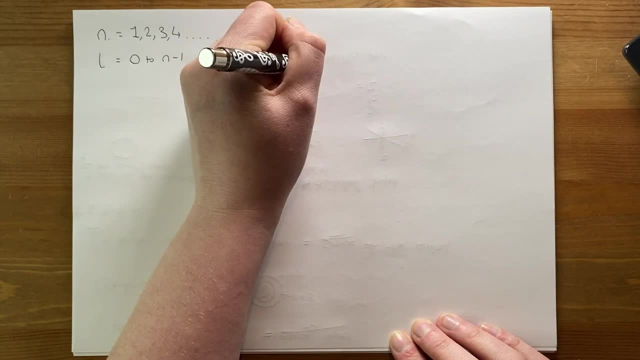 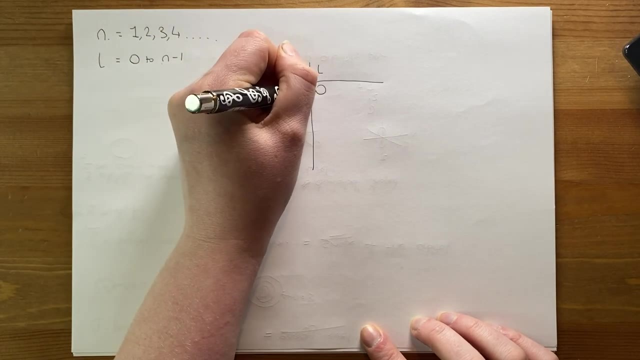 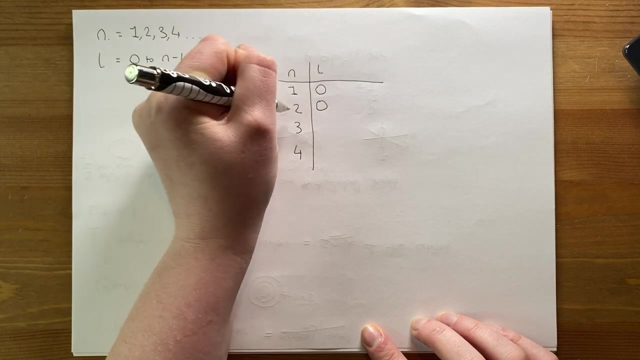 1,, 2,, 3, or 4,. l can go from 0 to n minus 1.. So 0, n minus 1 is 0.. There can only be one shape Here. this can go 0.. 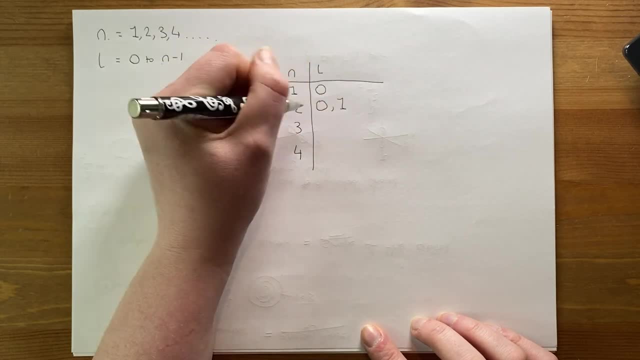 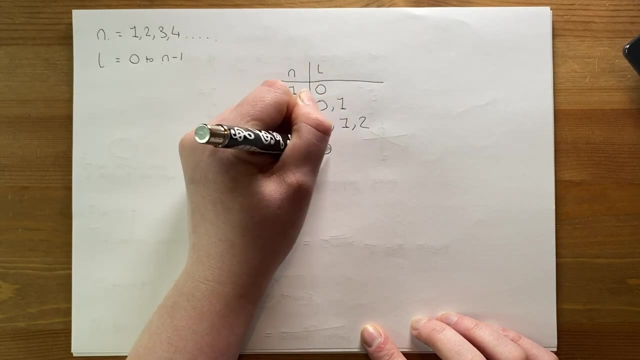 It can also go to 1.. It can't go to 2,, because 1 is n minus 1.. Here it can go 0, 1, 2.. Here I can go 0, 1, 2,. 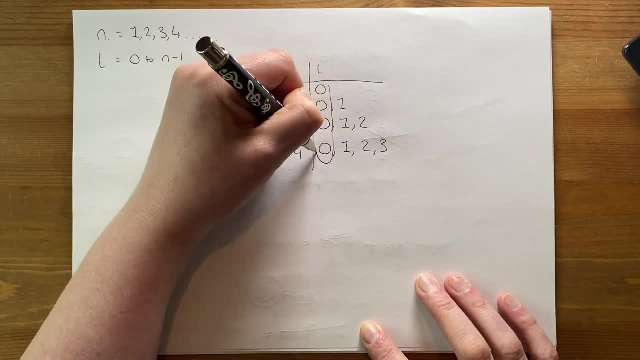 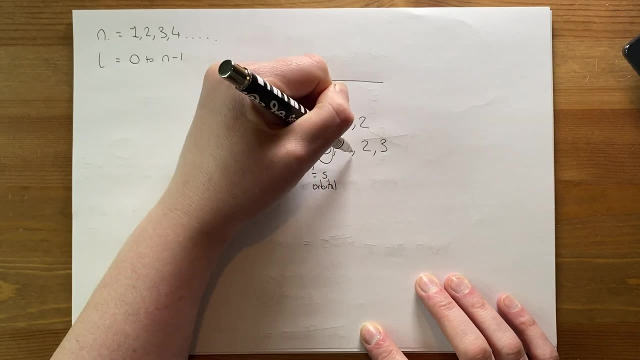 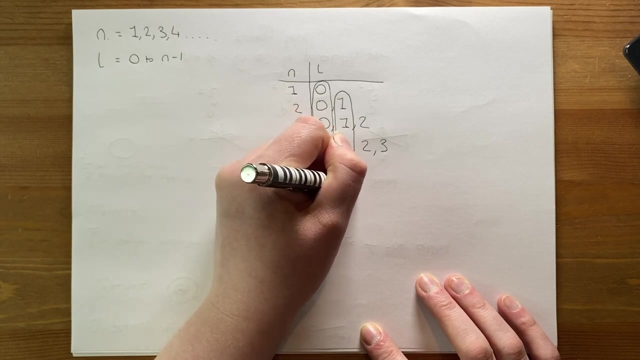 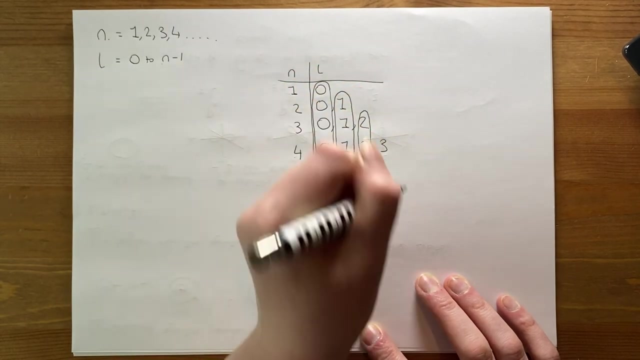 and 3.. This might seem confusing. This: if l equals 0, that equals an s orbital. If l equals 1, that equals p orbital. I'll put that here. If that equals 2,, that equals d orbital. 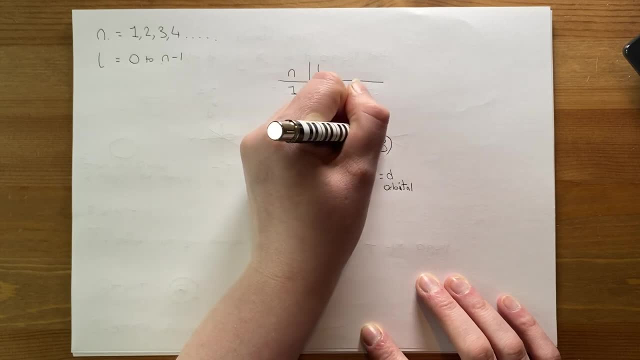 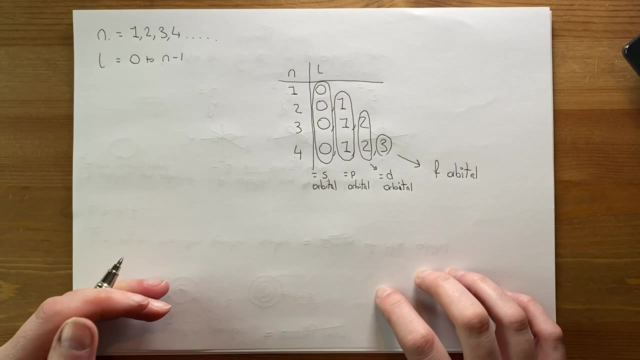 Oh, I cannot spell this, do I? And if it equals 3, that equals something called an f orbital, Which we don't need to know the shapes of. We just they are funky shapes. You just need to know that they exist. 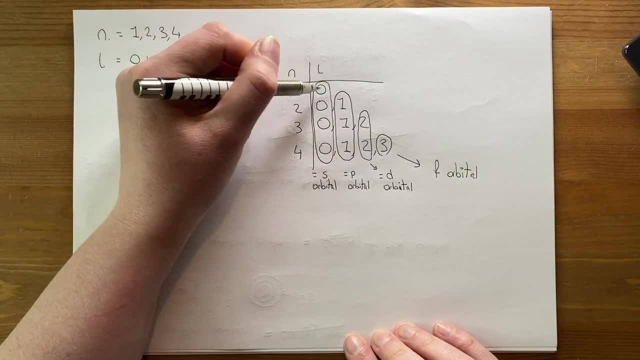 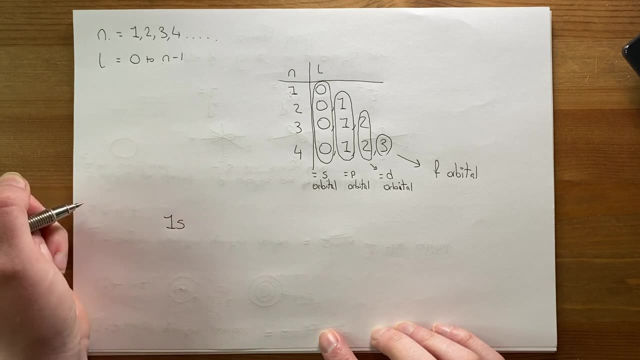 So I have my principal quantum number. In the first shell I can only have an s orbital, Can't have anything else. So in the first shell you can have 1s. That's how we would represent it If I had a second shell of electrons.